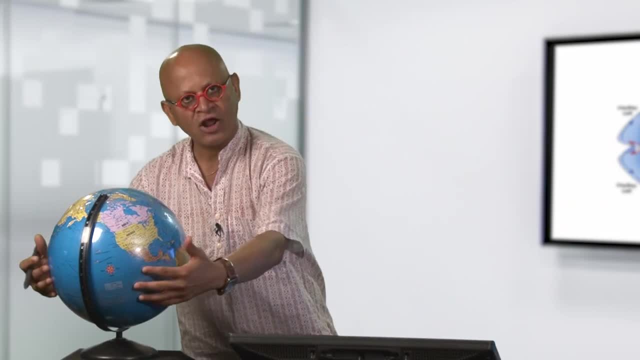 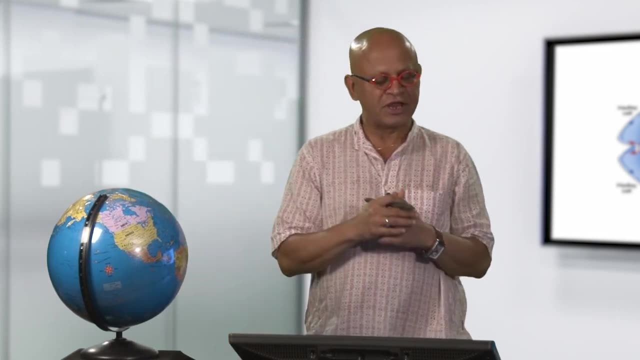 new air has to come in. So if the air is rising all around the equator, where can the air come from? it can only come from the north and south. There are other details which we will get into later on, but for now let us just assume that the tropics are uniformly being warmed. 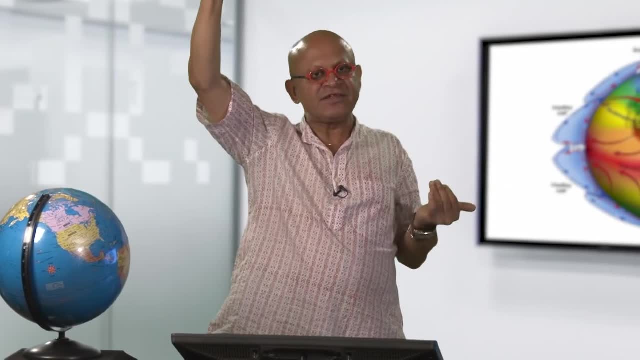 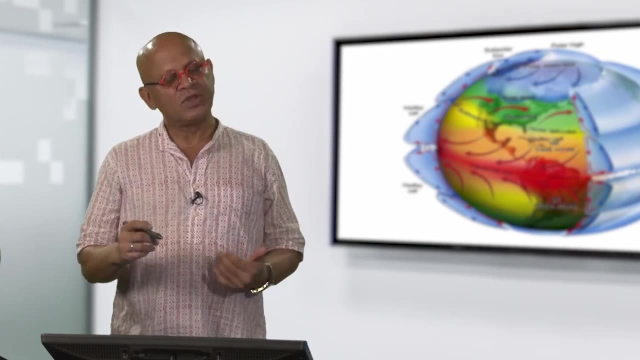 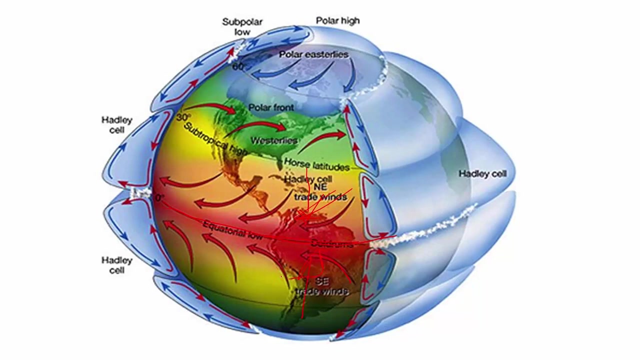 the air is uniformly rising from the surface. Air is coming into the equator to replace the rising air from the north and from the south. okay, So you remember your coriolis. now, If the air is coming from the north towards the equator and from the south towards the equator, what will coriolis do to it? Obviously, 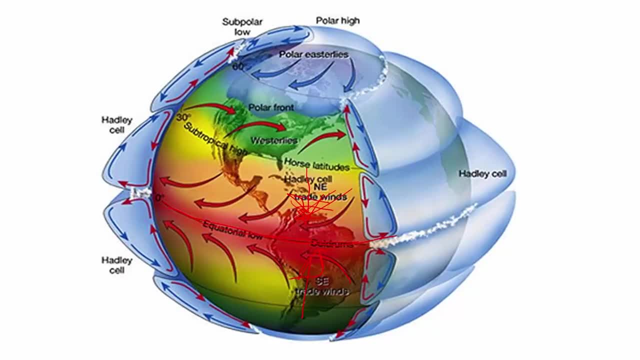 in the northern hemisphere, coriolis will tilt the winds to the right of the direction of motion. In the southern hemisphere, the coriolis will tilt the winds to the south. So in the northern hemisphere, the coriolis will tilt the winds to the right of the direction of. 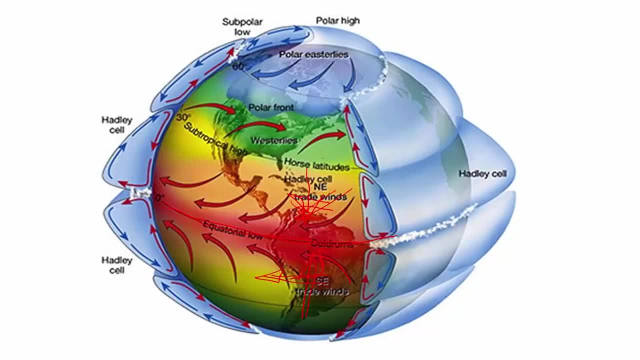 motion, which means the winds that are coming from the south will become south easterlies, which means they appear like they are coming from the south east. The winds that are coming from the north will become tilted and will become north easterlies. So they are coming. 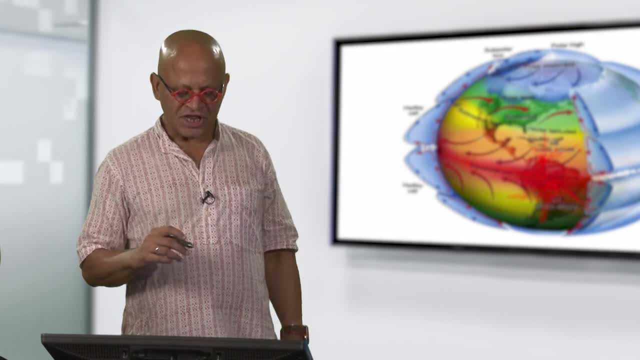 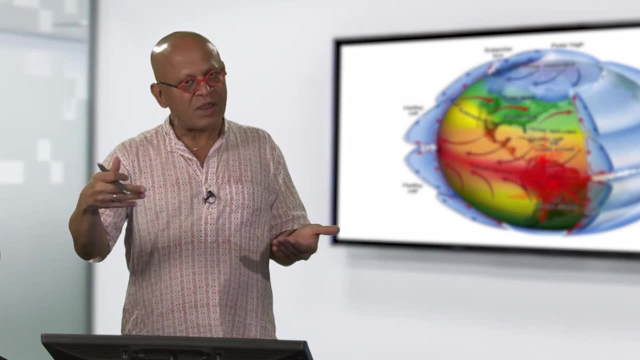 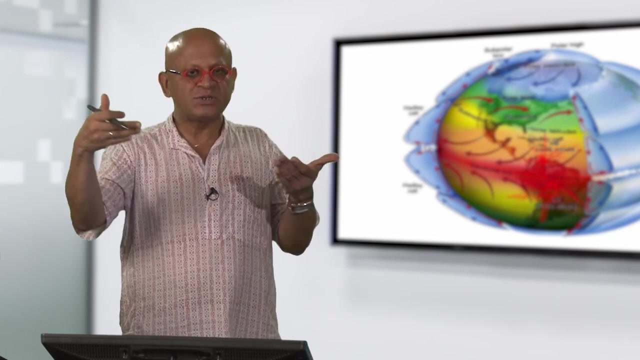 from the north east towards the south east. So essentially, this heating of the tropics- Imagine that are new air compensate for this. rising air creates this so-called convergence into the equator. So the air that's flowing from the north and south into the equator. 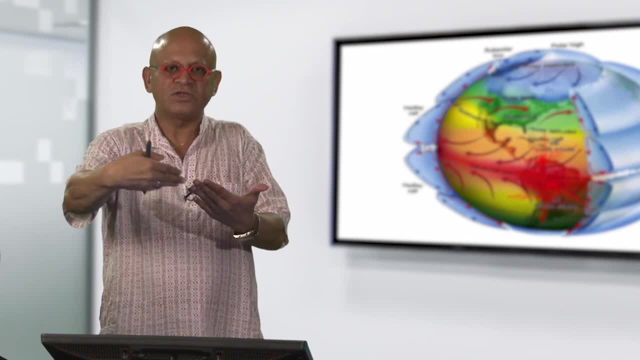 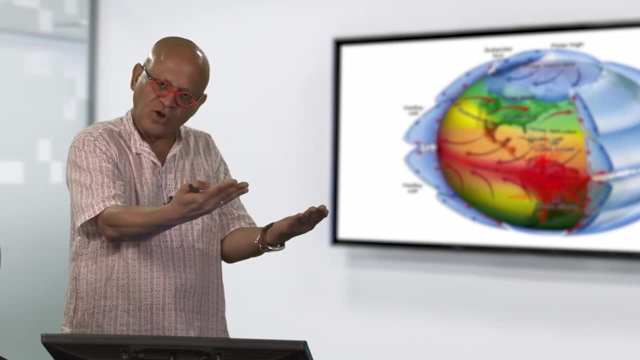 is called convergence. You add coriolis to the air that is converging towards the equator and you end up getting these straight winds that are north easterlies and south easterlies, And we already learned that the north easterlies and south easterlies requiresLETM's. 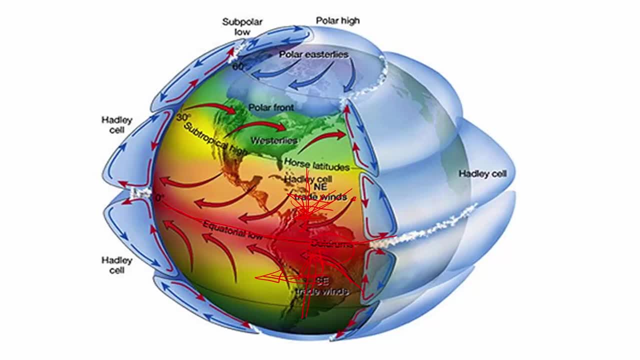 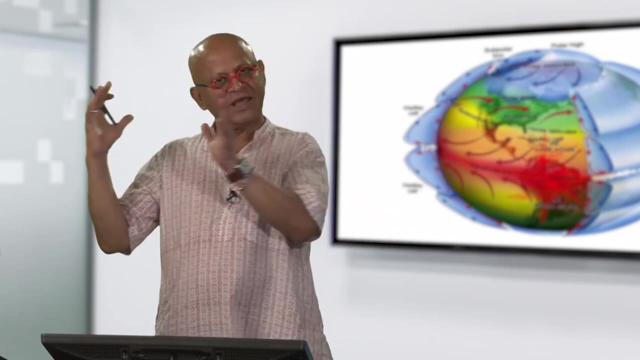 January 14, 2015, forcing the water away from the equator and creating upwelling. So, essentially, then, you have to put in your continents, create individual oceans like the Pacific Ocean, the Indian Ocean and the Atlantic Ocean, and see in each ocean what